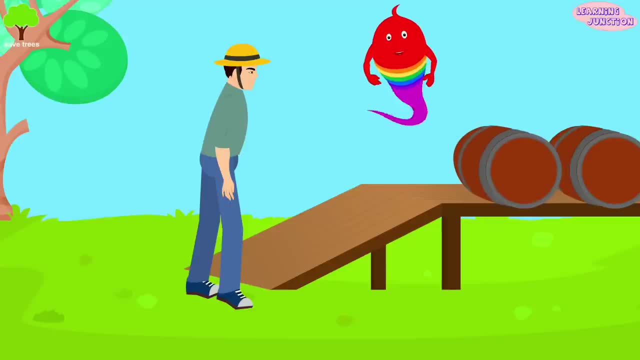 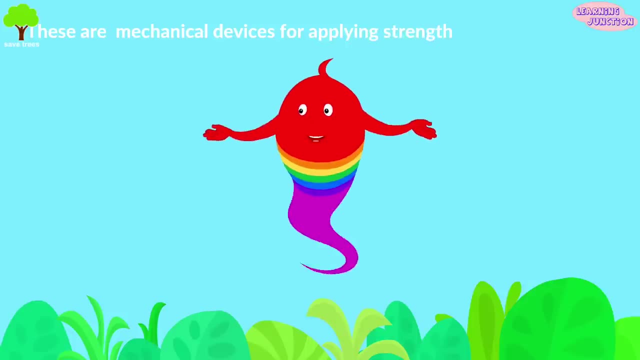 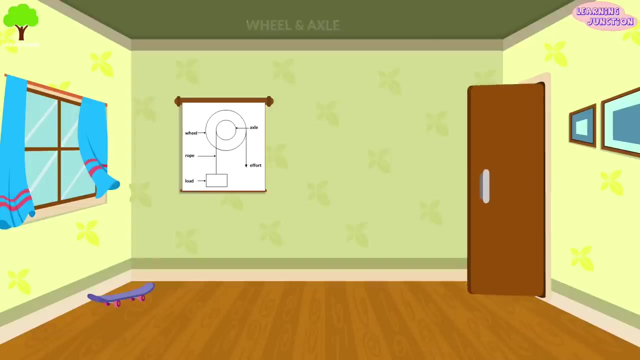 using a simple machine, an inclined plane. simple machines are very basic mechanical devices for applying strength and performing work. let's see six different kinds of simple machines: wheel and axle. it makes work easier by moving the objects across distances. the wheel turns with the axle, causing movement. an 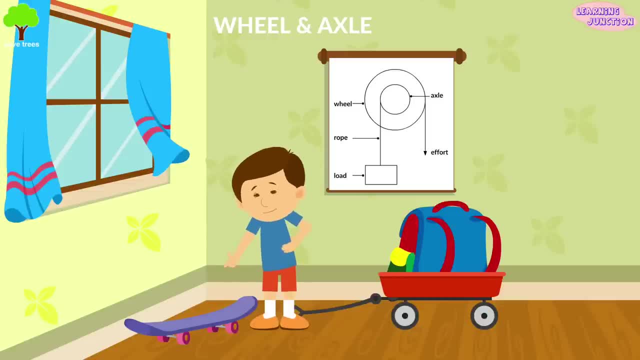 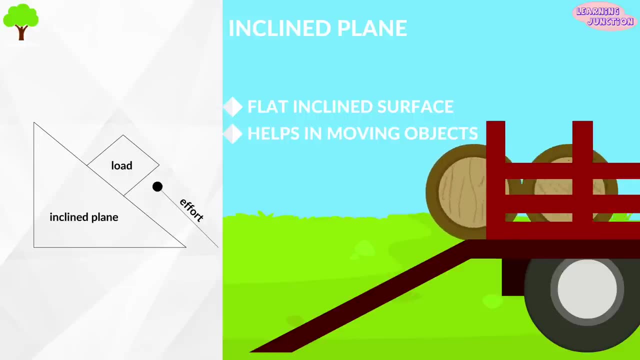 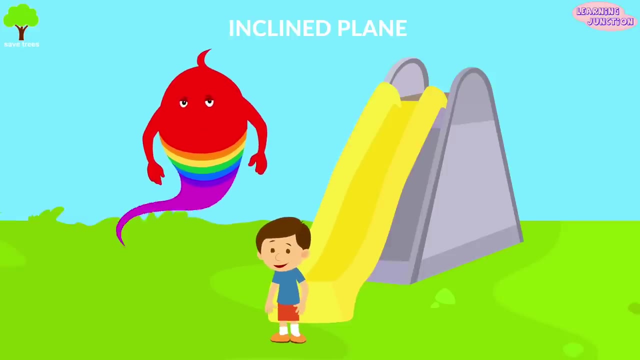 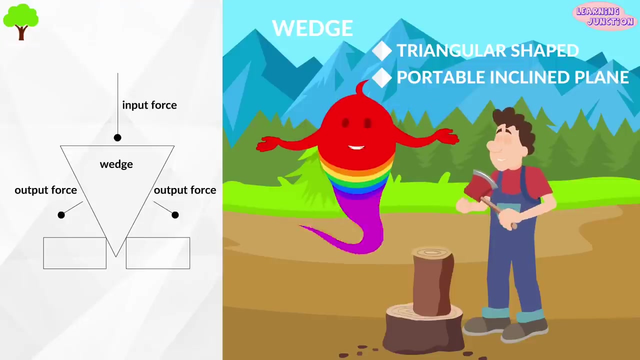 example is your skateboard inclined plane. it is a flat surface that is inclined so it can help move objects across distances. aha, this slide is also an example of inclined plane wedge. a wedge is a triangular shaped tool and is a portable inclined plane. it can be used to separate two objects. lift up. 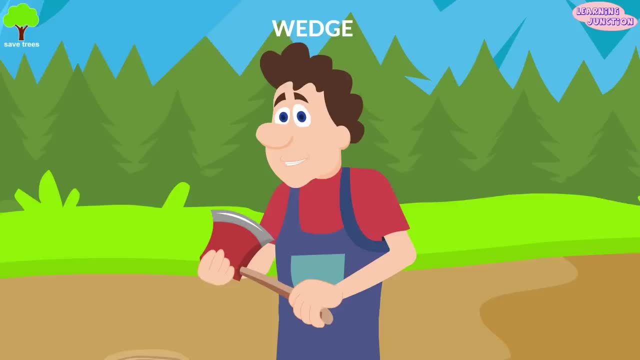 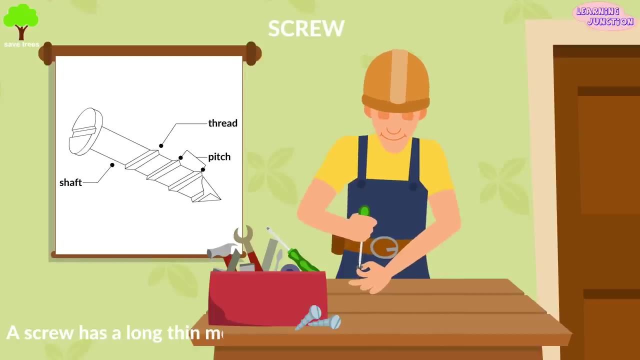 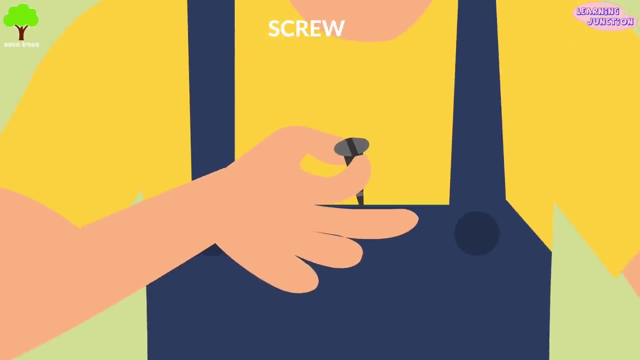 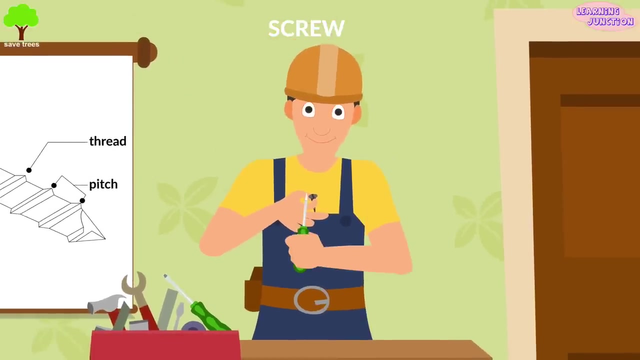 an object and hold an object in place. an axe blade is an example of a wedge screw. a screw has a long, thin metal shaft with threads spiraling along its length. it also has a turning head with a groove where a screwdriver can be used to rotate the screw. it can be used to lift things or to hold things together. 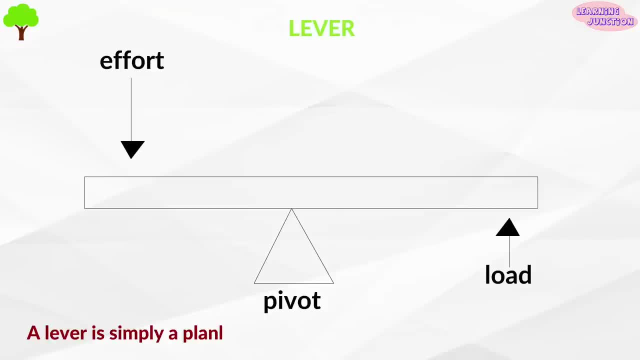 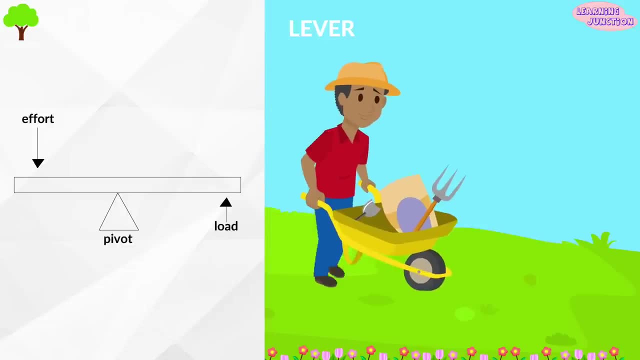 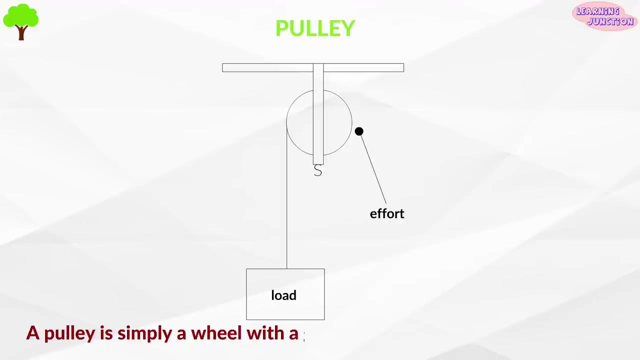 lever: a lever is a tool that can be used to rotate a screw or to hold things. is simply a plank or ridged beam that is free to rotate on a pivot. it is perfect for moving or lifting heavy things. pulley: a pulley is simply a wheel with a. 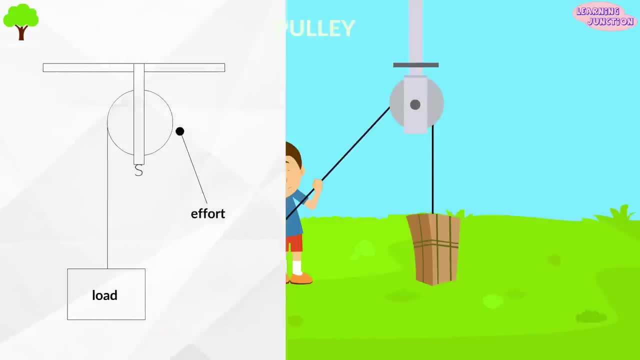 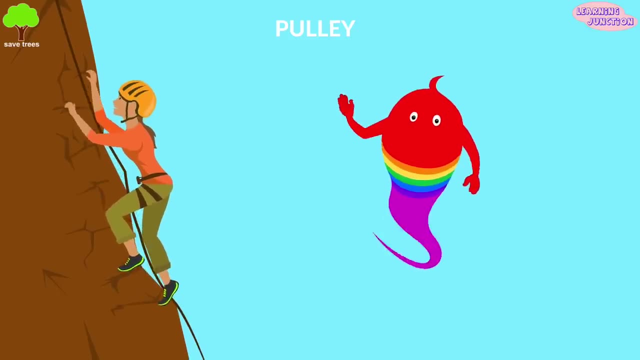 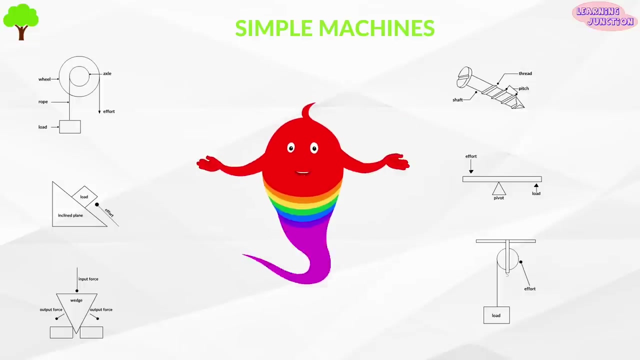 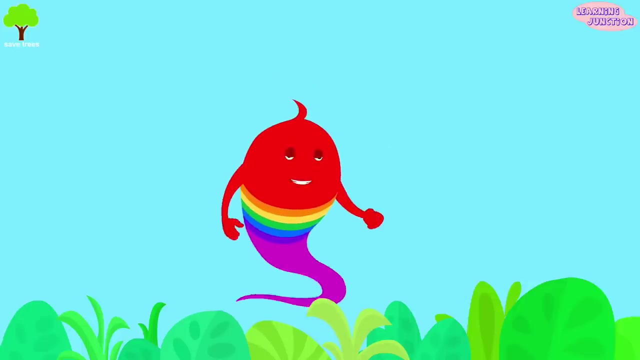 groove in it and a rope in the groove. it is used to lift up or lower heavy objects. with the help of the pulley system, rock climbers can climb steep rock surfaces easily. here's a chart of various simple machines: wheel and axle inclined plane, wedge, screw, lever, pulley. now you know a lot about simple machines. please drop a. 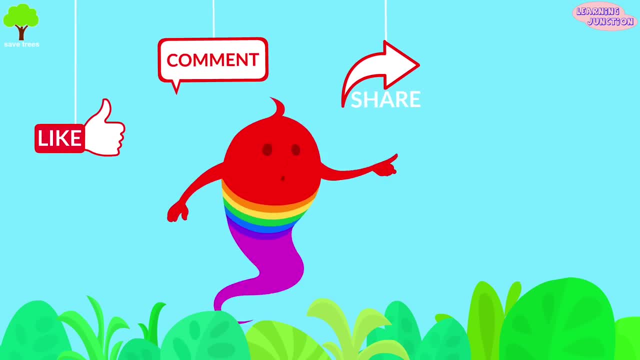 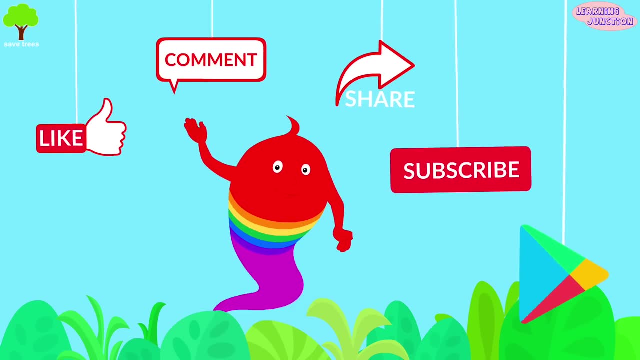 like, leave a comment, share the videos and don't forget to subscribe. our app learning Junction is available on Play Store. bye, bye.